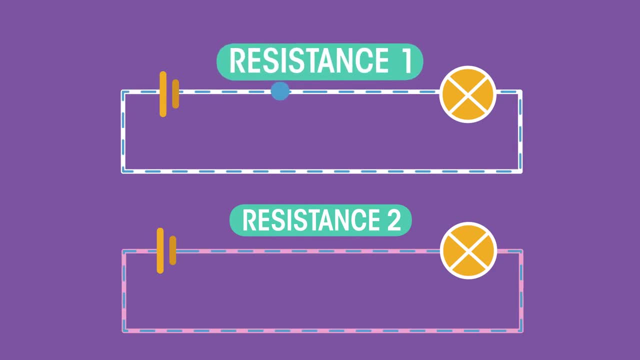 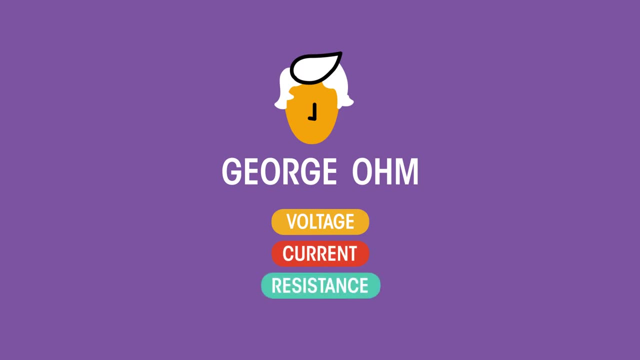 voltage to move electrons through it, compared to one of a lower resistance. George Ohm found a relationship between voltage, current and resistance in a circuit which we know as Ohm's law. V equals I times R. R is the resistance measured in ohms, V is voltage measured in. 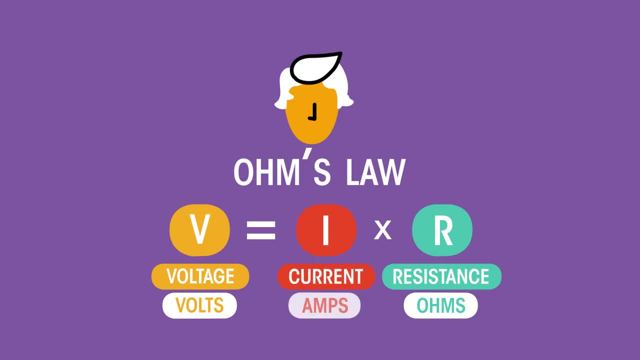 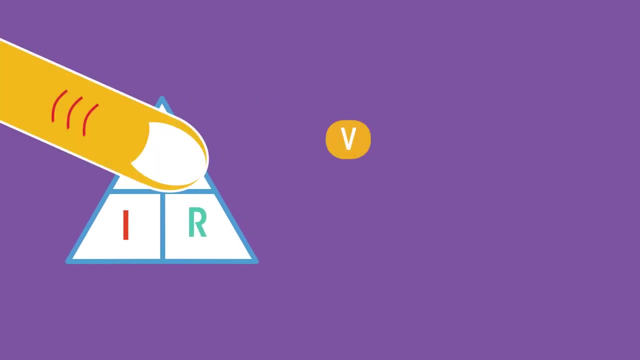 ohms and I is current measured in amps. Thus, for a particular wire, if you want to double the current flowing, you need to double the voltage applied. Ohm's law can be displayed in a formula triangle like this: Voltage equals current multiplied by resistance. Current equals voltage divided. 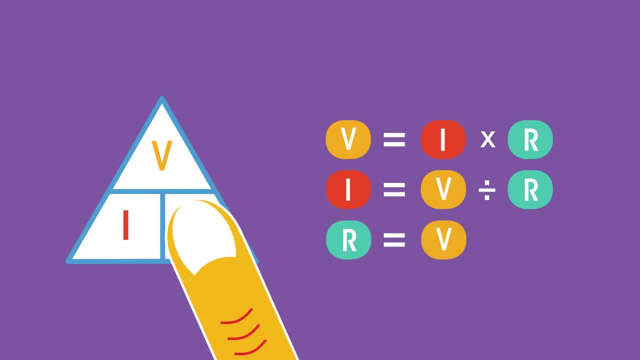 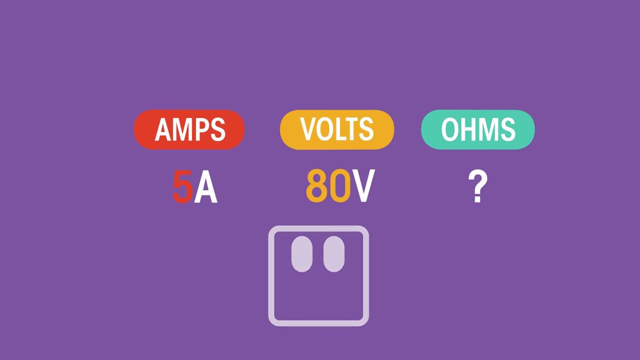 by resistance, and resistance equals voltage divided by current. Let's try an example. A wire is carrying a current of 5 amps with a potential difference of 80 volts across it. What's the resistance of the wire? Pause the video for a moment and have a go. 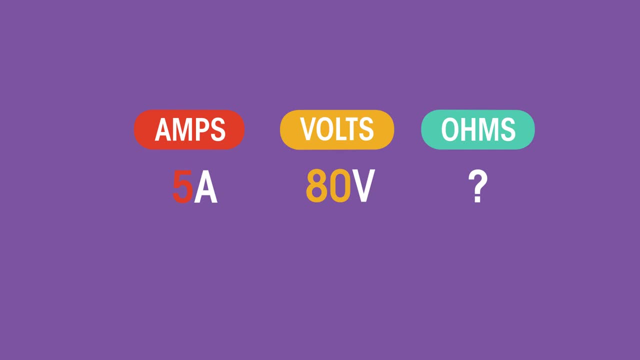 We should use the equation: R equals V over I, which equals 80 volts over 5 amps, which equals 16 ohms. Remember: resistance is measured in ohms. Ohm's law is measured in ohms. Ohm's law is measured in ohms. 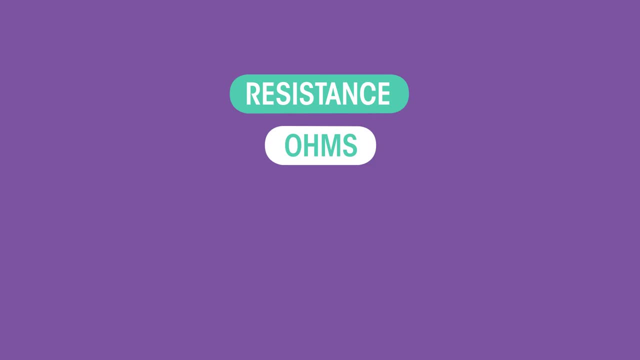 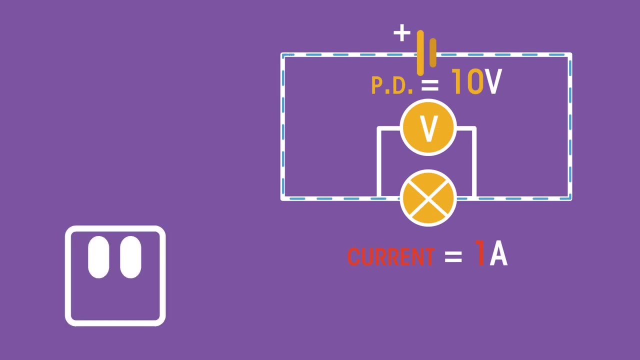 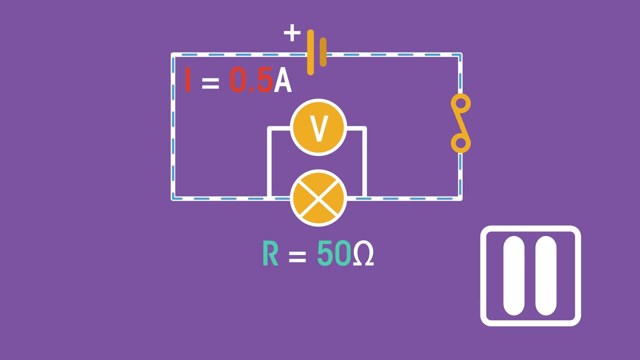 And the symbol for this is omega. Let's try two more examples. Calculate the resistance of the lamp in this circuit. Pause the video while you work out the answers. Calculate the voltage or potential difference across the lamp. Did you get them right? 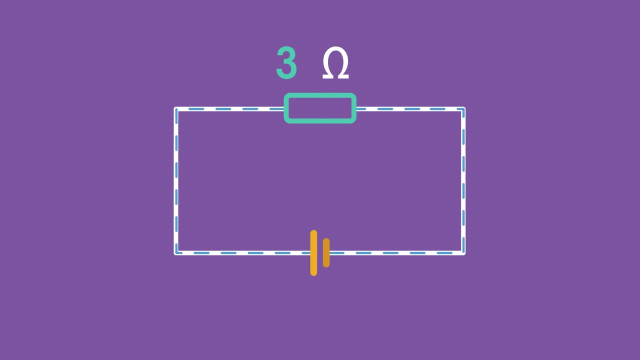 You also need to know that the resistance of a conductor increases as its temperature increases. This is because temperature is a measure of the vibration of the atoms within the conductor. As the atoms vibrate more, so the electrons collide more often, making it more difficult for the electrons to flow and so increasing the resistance. 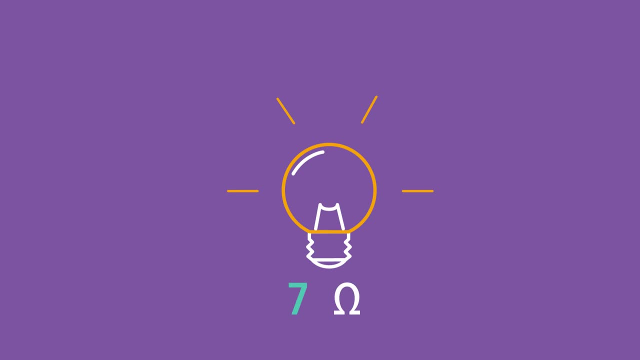 Thus the resistance of an old-fashioned filament bulb increases as the filament gets hotter and hotter. So that's how resistance happens in a circuit and how it can be calculated.